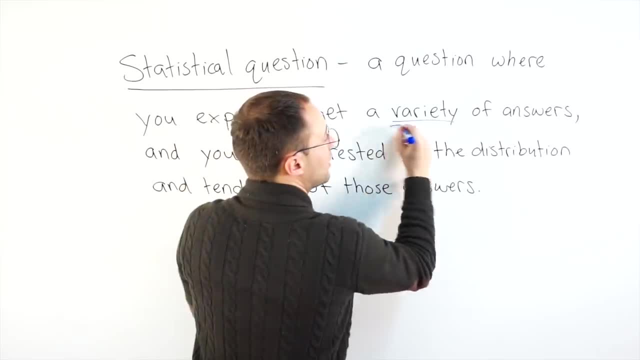 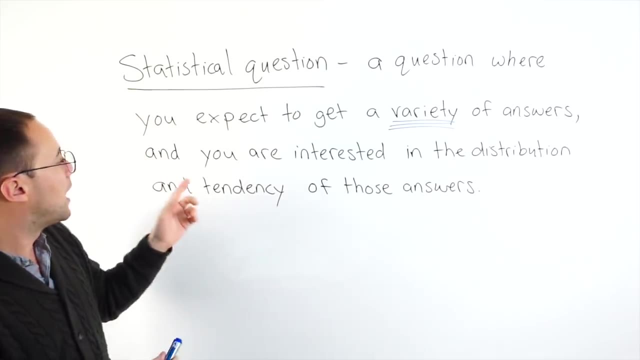 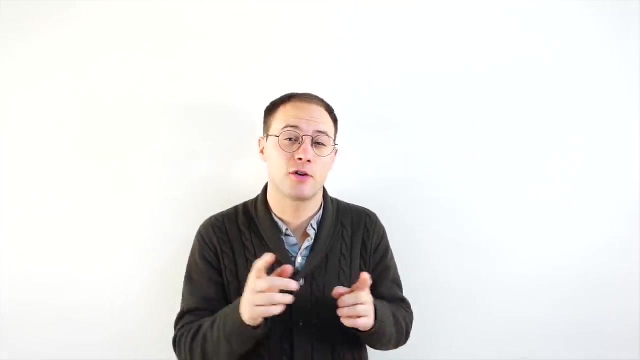 That's really big: A variety of answers, A whole range of answers. You're not expecting just a couple of different options, right? And you're interested in the distribution and tendency of those answers. Now one more thing I want to add about statistical questions. 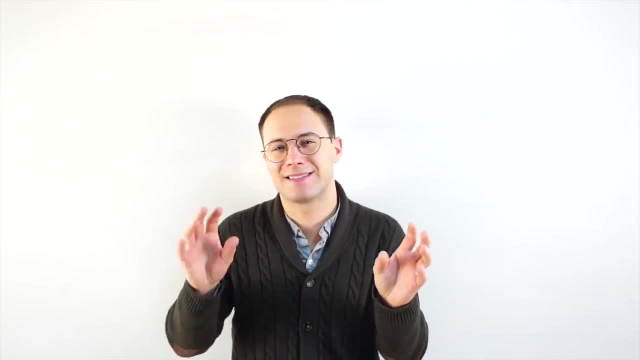 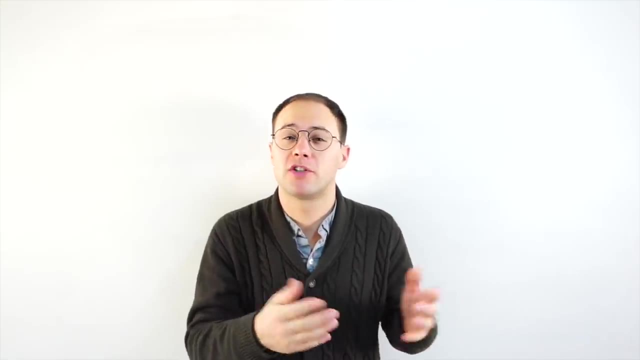 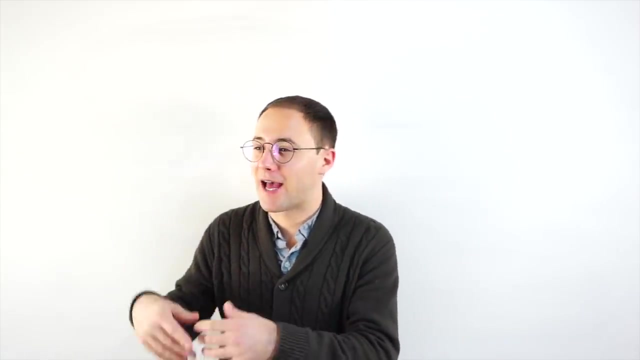 Don't get confused from a survey question and a statistical question. For example, if your statistical question was how much do sixth graders weigh? Well, that's a good question. Well, that's your statistical question. But when you do the survey, you're not going to ask people. 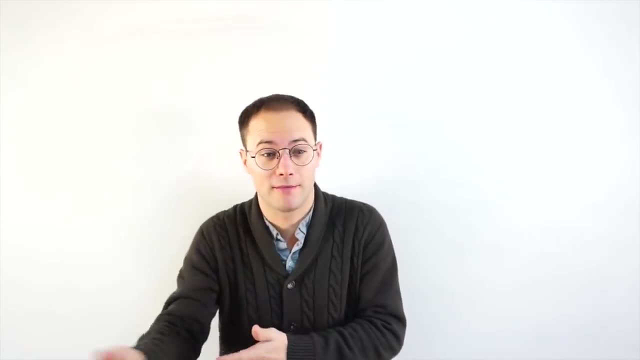 how much do sixth graders weigh? You're going to say how much do you weigh And you go to the next person- how much do you weigh? And all the sixth graders you're going to survey. you ask them: how much do you weigh? 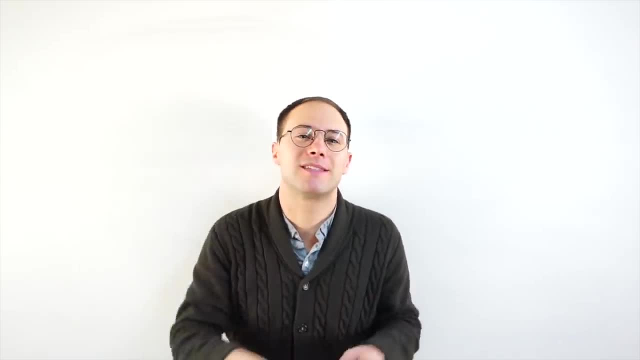 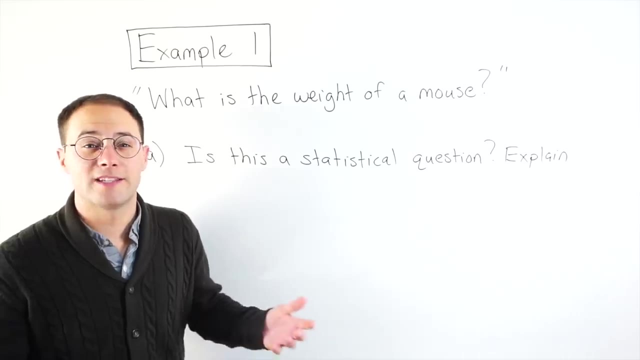 That would not be a statistical question, but it's going to help us get data to answer the statistical question. So with that let's get to our first example. Okay, example one. Let's say your science teacher asks you to do an experiment. 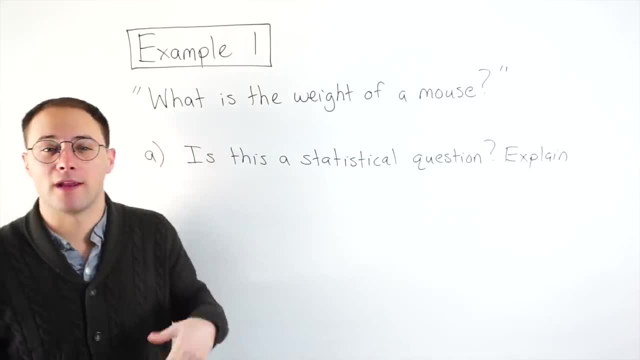 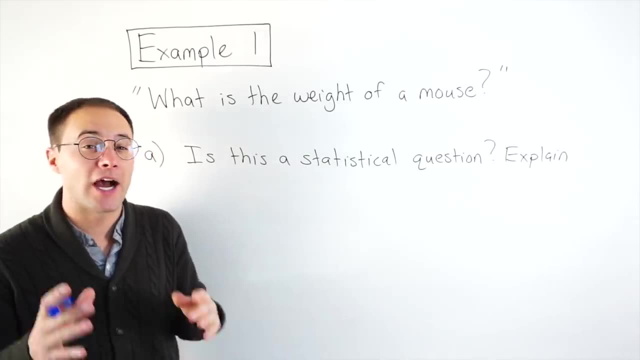 about what you think is a good statistical question. And she asks: what is the weight of a mouse? Well, first, is this a statistical question? And if so, explain Now, if you remember from the definition, statistical questions should be giving us a variety of answers. 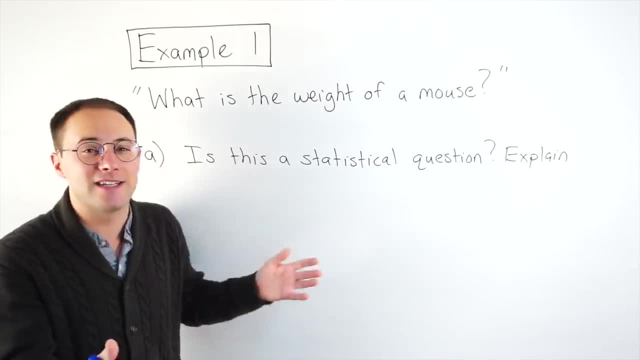 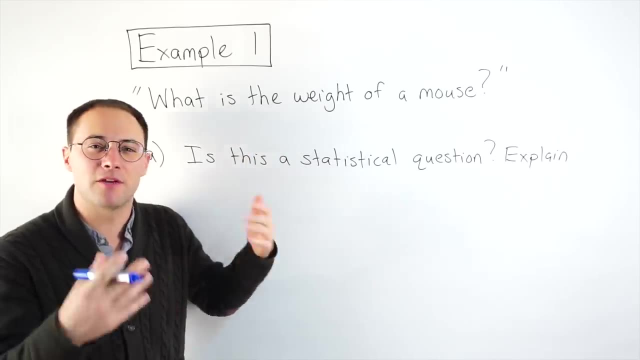 They should be able to show us a distribution and a tendency. So we have to think well, this question: if I'm doing an experiment with mice, is it going to give me a variety of answers? And the answer is yes, it will. 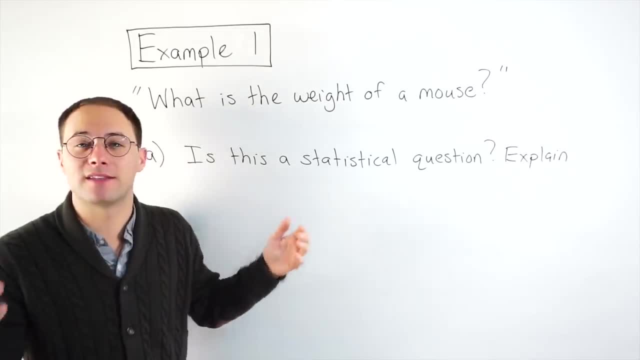 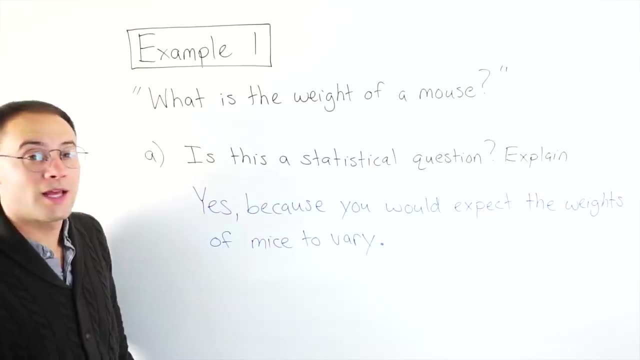 because you can't expect all mice to weigh the same. They're going to be different, just like humans are going to weigh different amounts, same with mice. So our answer: yes, because you would expect the weights of mice to vary. Let's try part B. 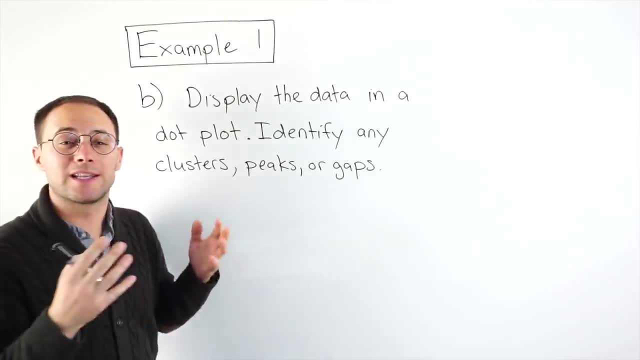 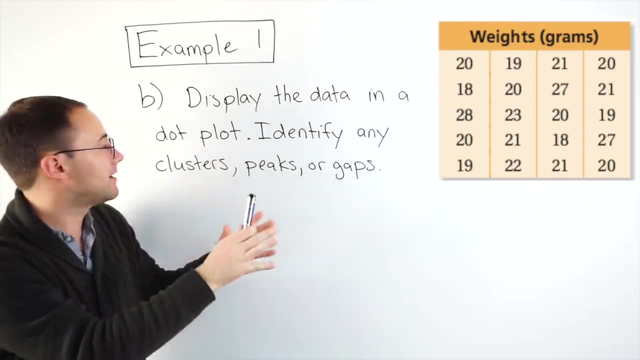 Okay, part B. So we weighed a whole bunch of mice and we collected that data and have it in this little table over here. Now what we're going to do is display that data in a dot plot, So it looks kind of confusing. 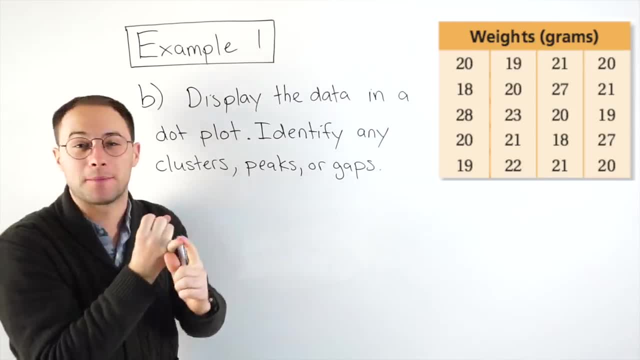 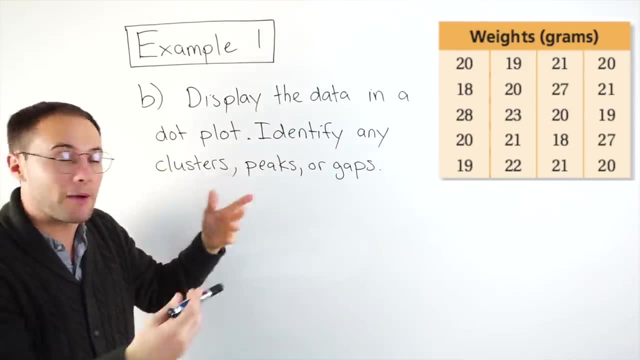 It's hard to tell anything about the data. right, We've already done that first step, collecting the data. Now we're going to organize it and we're going to make a dot plot. And then, after the dot plot is made, 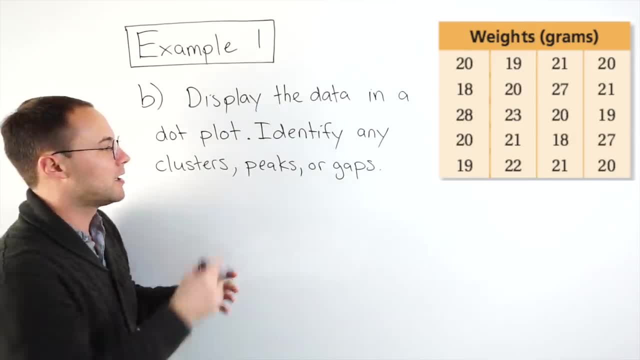 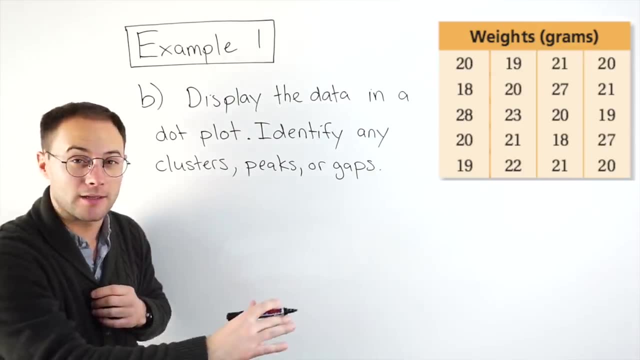 identify any clusters, peaks or gaps, And we'll talk about what those mean in a second, But first the dot plot. A dot plot is basically you have a number line- It could be a horizontal or vertical- And then you use dots to show where the different data 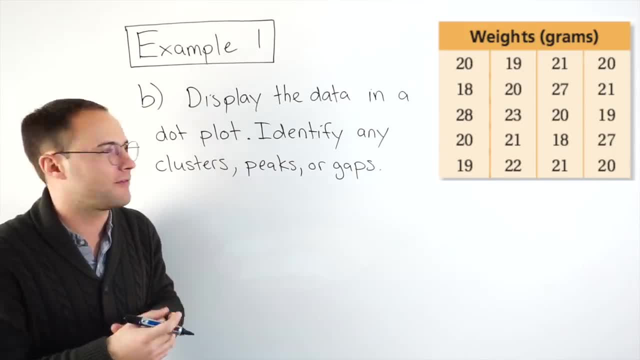 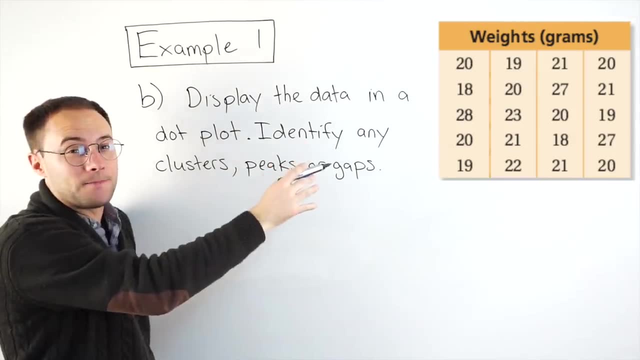 values are. It's kind of like a little bit like a bar graph, except with dots instead of bars. So we're going to start with a number line. Well, if I look at my data, I can see that the least value is 18,. 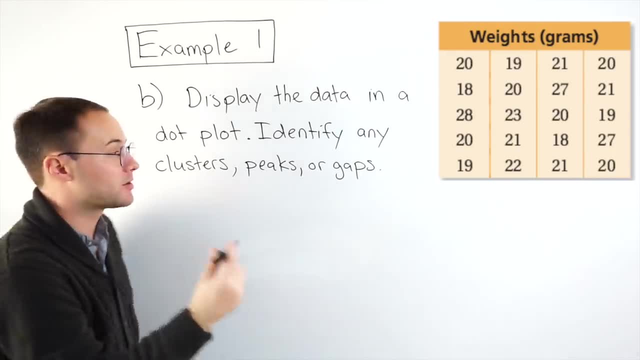 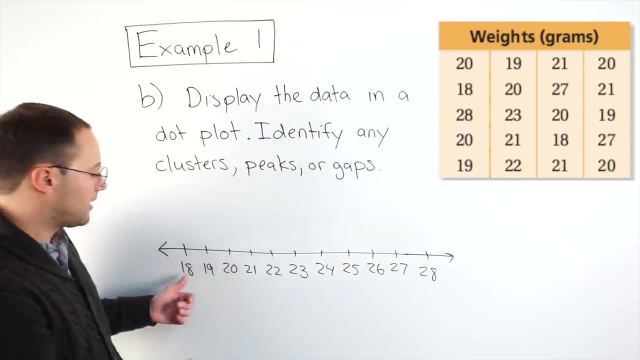 18 grams and the greatest was 28 grams. So that's where I'm going to start on my dot plot. Okay, so I have my number line done for my dot plot, all the way from 18 to 28.. I need to label. 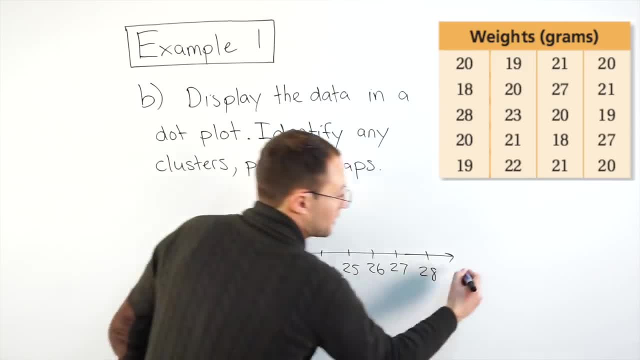 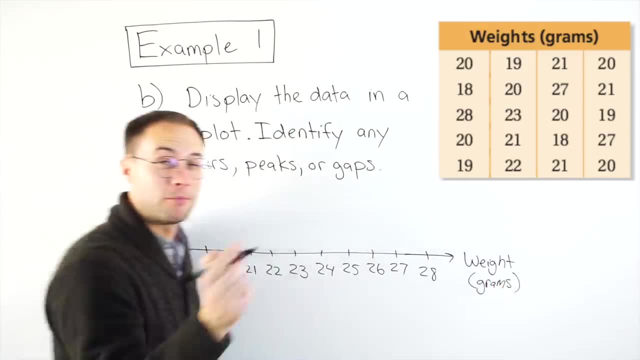 What these values mean. So these were all weight, So I'm going to label that over here to the side Weight. and that was in grams, Really important to label. Don't forget that, or else nobody's going to know what those values represent. 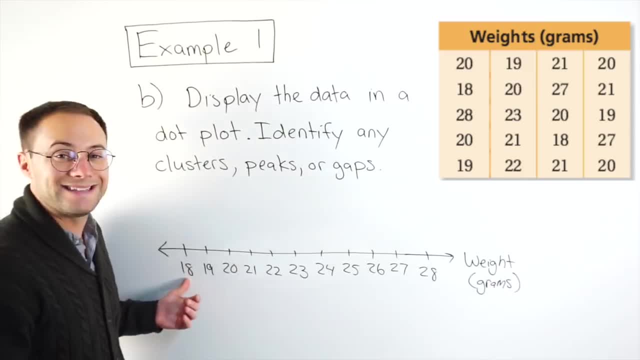 And then we just look at the data and put dots. So at 18,, how many mice weighed 18 grams? Well, if I look at my data, I can count two. So I put one, two, just two dots right above that number 18.. 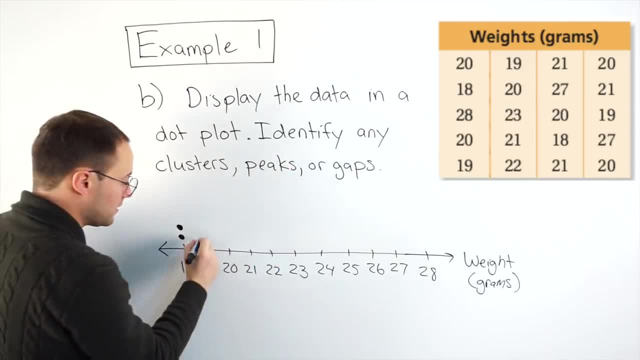 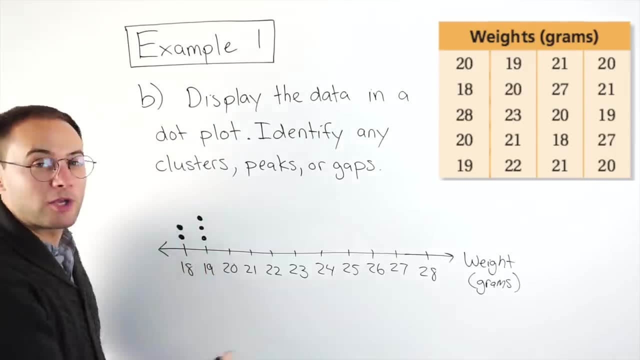 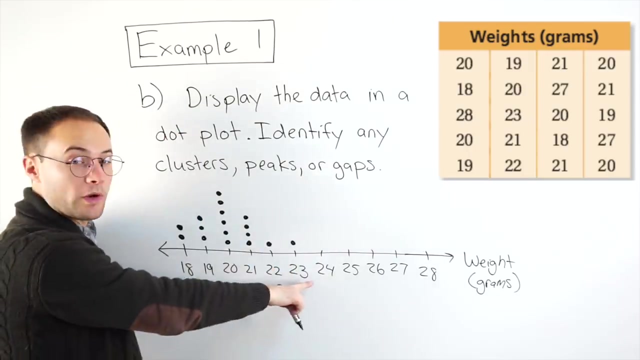 And I keep going, So 19,. if I look, there were three, So I'm going to do one, two, three like that And we'll keep going. At this point you'll notice there were no 24s, no 25s, no 26s. 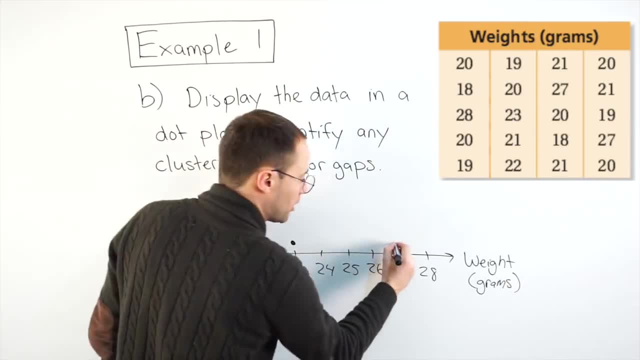 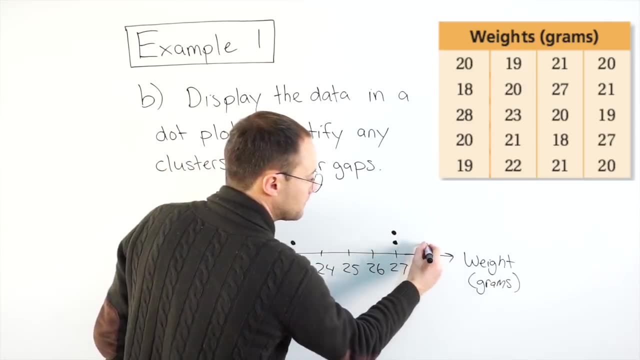 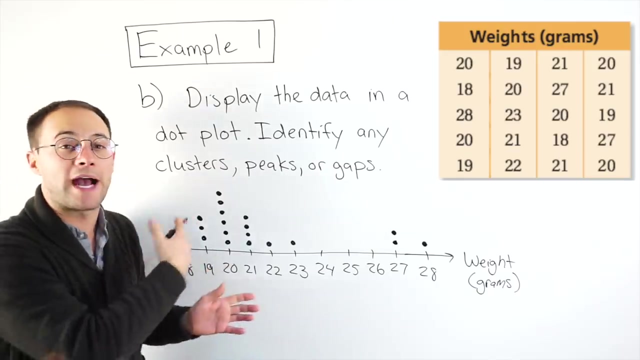 So I'm going to put nothing there. And then I get to 27 and keep going. So there are two of those And then finally one, 28.. One good thing to do before you're finished is just double-check to make sure you've counted. 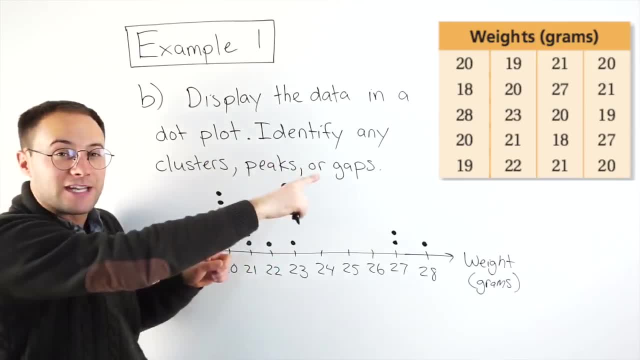 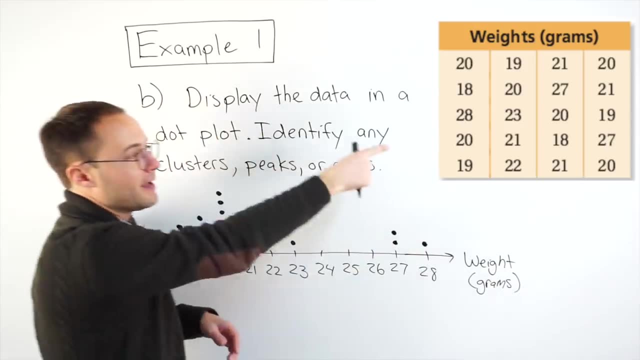 all of the data values. So just count your dots and make sure it matches the values over there. So I've got one, two, three, four, five, six, seven, eight, nine, 10,, 11,, 12,, 13,, 14,, 15,, 16,, 17,, 18,, 19,, 20.. 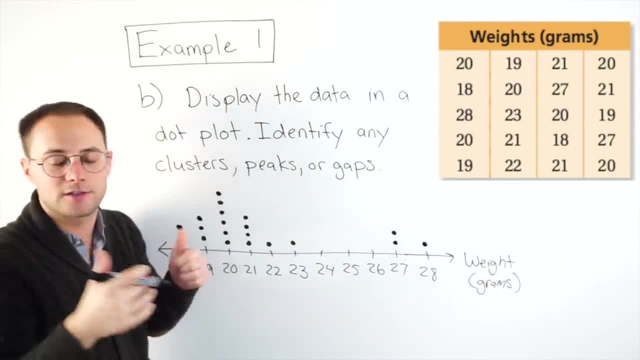 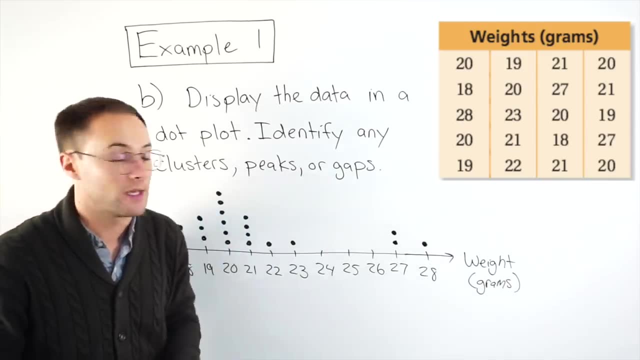 And if I look at that little chart, I have 20 values there, So I'm happy with that. Now dot plot is done. Let's go to the next part. Identify any clusters, peaks or gaps. Well, let's look at the clusters. 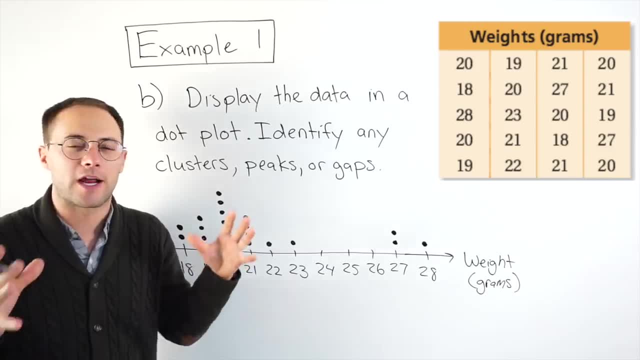 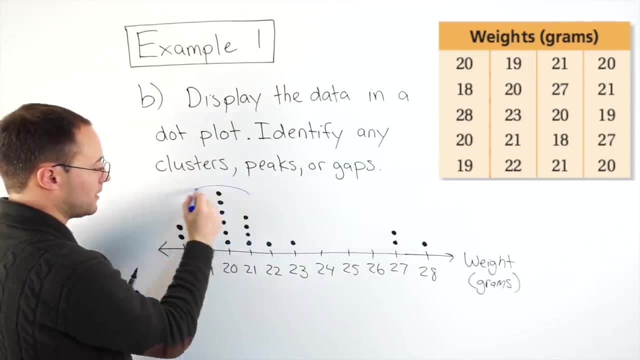 First, a cluster is where a lot of data values are kind of bunched together. So if you look over here you'll notice, well, it looks like there's a whole bunch of data values right there. You're just going to pick kind of what's in the middle. 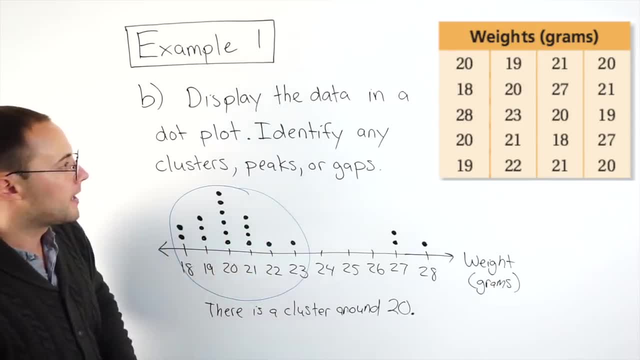 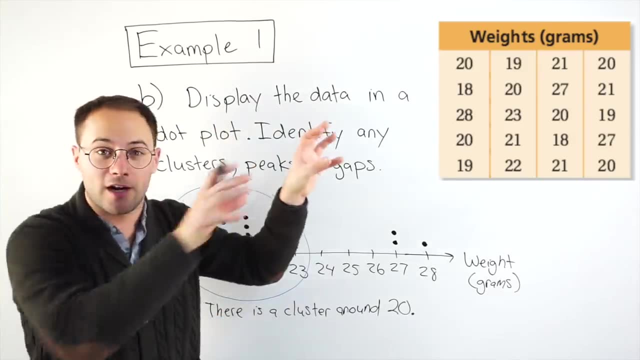 where they're kind of all seem to kind of be drawn to. So that would be 20.. So that's a cluster. You might be asking. is it possible to have two clusters? Sure, If you've got a big bunch here and another big bunch here. 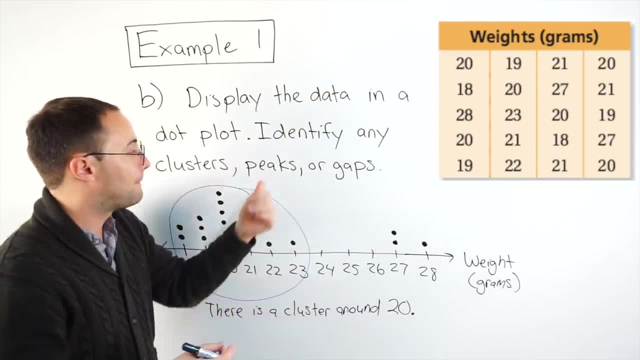 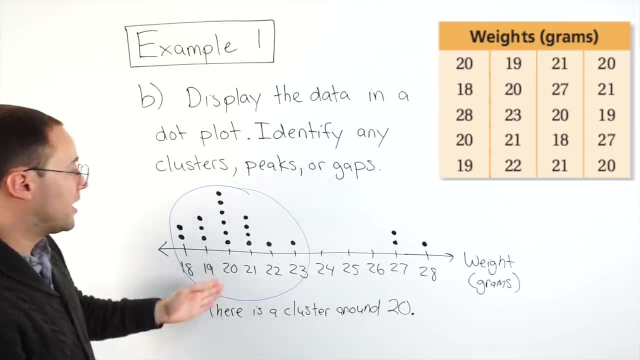 it's possible to have more than one cluster, That's OK. Peaks: well, hopefully you can kind of guess what that is. That's just, are there any things where it's the tallest? So, right here again, 20,. there is a peak at 20.. 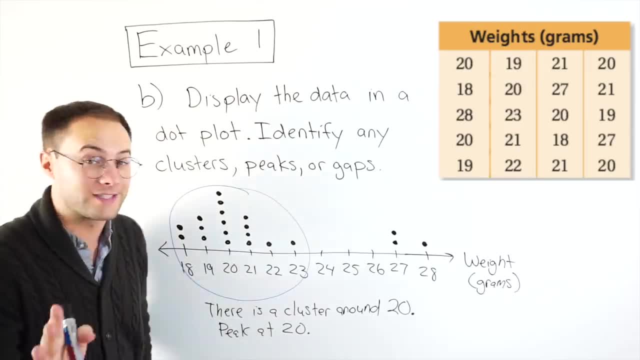 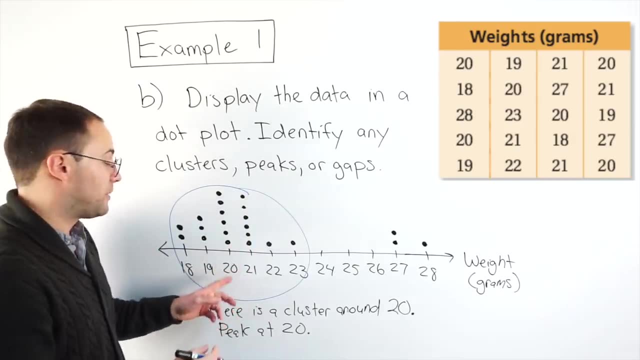 And same thing. it's possible to have more than one peak. If, for example, 21 also went up to six, then we would say there's a peak at 20 and 21.. But as of right now, there's only one peak. 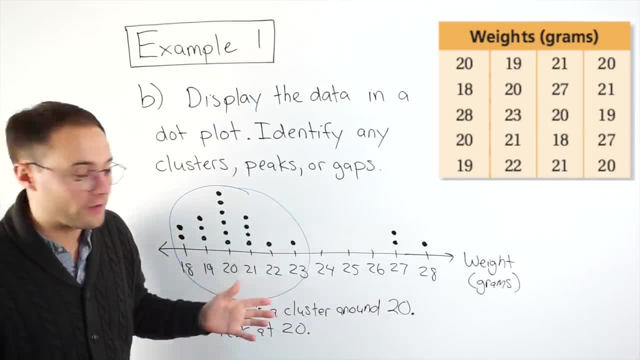 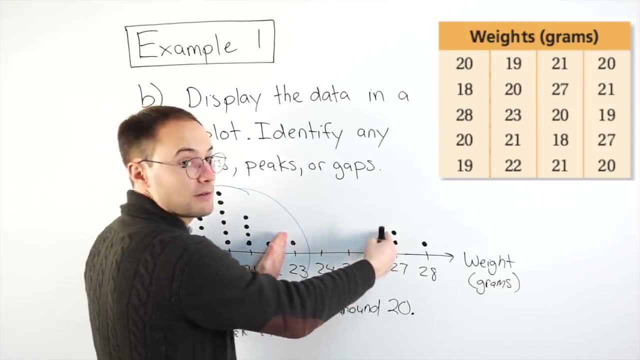 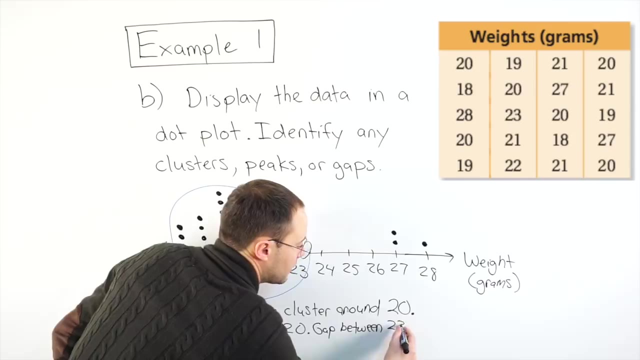 because that is the tallest. And finally, gaps. Hopefully that's obvious Again- what that is, where there's spaces in between the data values, and that obviously is right here. So there is a gap between 23 and 27.. 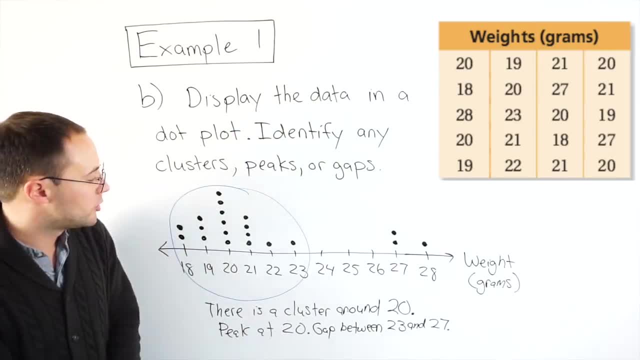 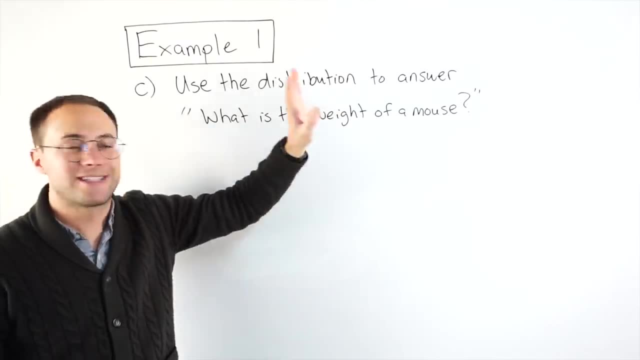 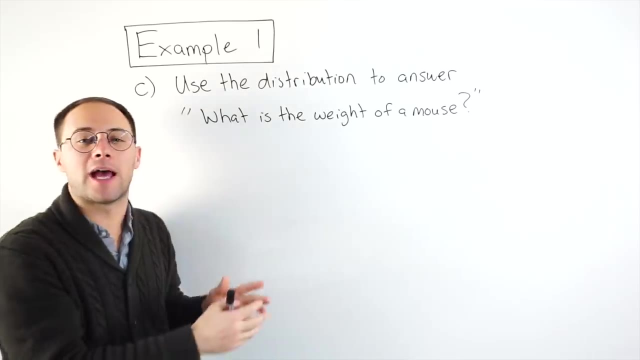 OK, So that's just kind of helping to examine and explain our data a little bit. more. OK, and finally, part C: use a distribution to answer: what is the weight of a mouse, our original statistical question. Well, looking at that data, looking at our dot plot, 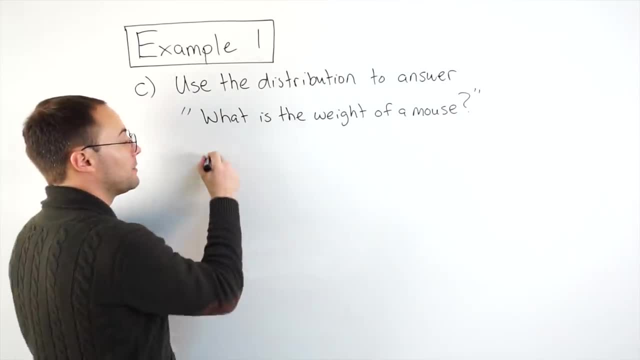 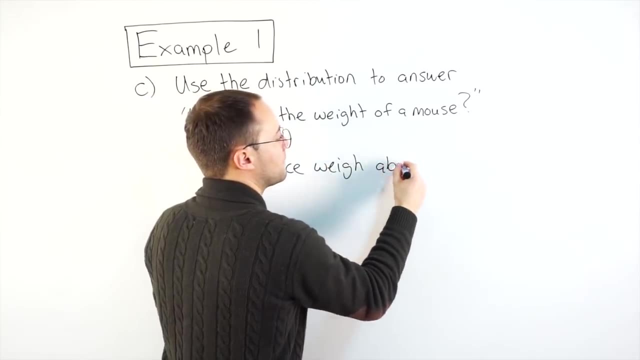 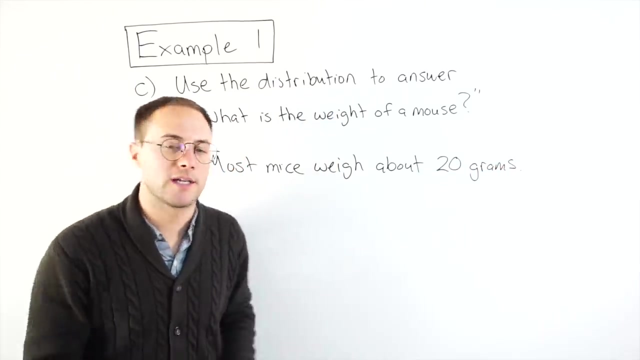 and seeing those clusters and the peaks, we can say that most mice weigh about 20 grams. Right, Our cluster was around 20.. Our peak was at 20.. So that's how we would answer that question. Here's one to try on your own. 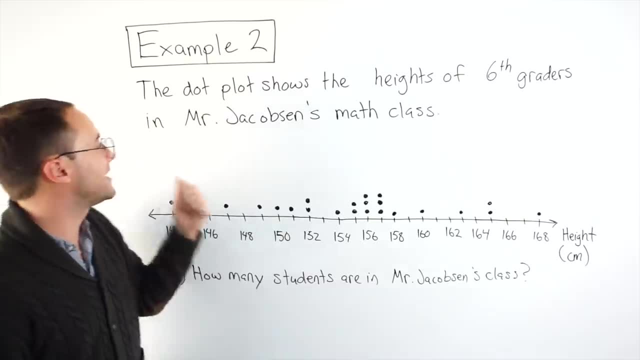 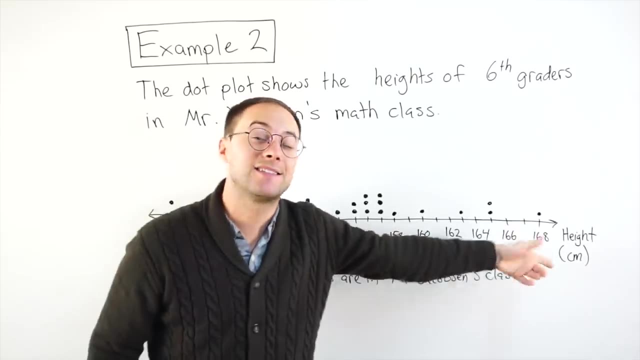 All right. example two: The dot plot shows the heights of sixth graders in my math class. So here is the dot plot. You can see these are all heights in centimeters, not inches, And part A says how many students are in my class. 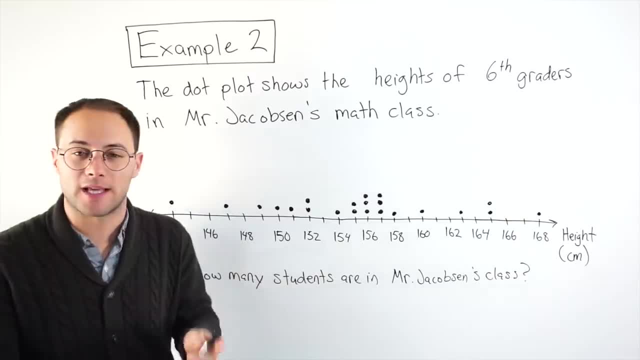 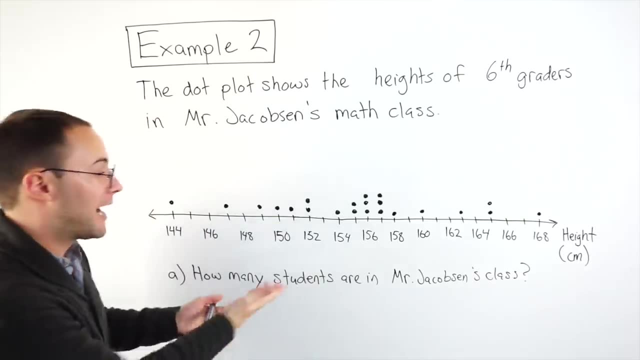 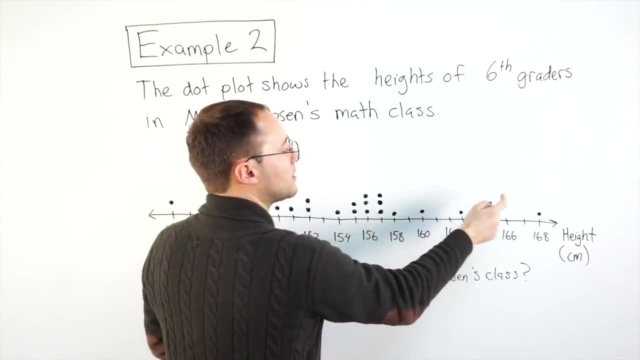 Well, if you remember, all of these dots represent a data value. So in this case, these dots represent one student's height. So to figure out how many students, I just count the dots. So let's see: we got 1,, 2,, 3,, 4,, 5,, 6,, 7,, 8, 9,, 10,, 11,, 12,, 13,, 14,, 15,, 16,, 17,, 18,, 19,, 20,, 21, 22.. 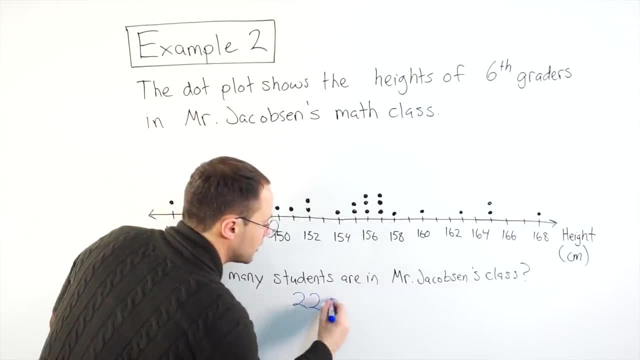 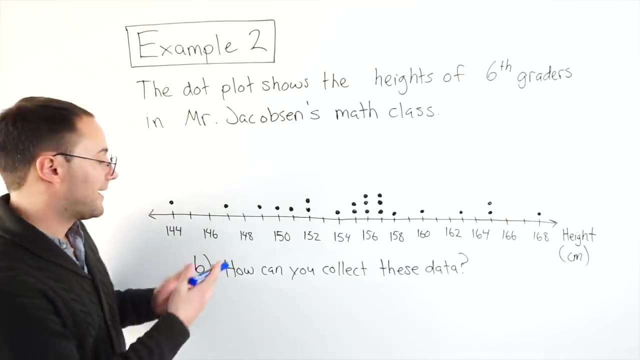 So there are 22 students in my class. OK, let's try part B. OK, part B. how can you collect these data? Well, to figure out heights, we're probably going to use a measuring tape, right? And make sure that you're measuring in centimeters, right? 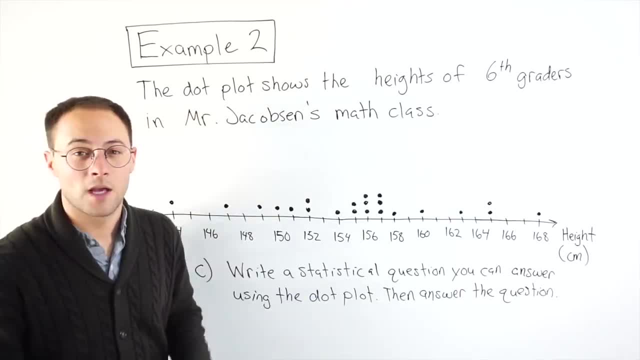 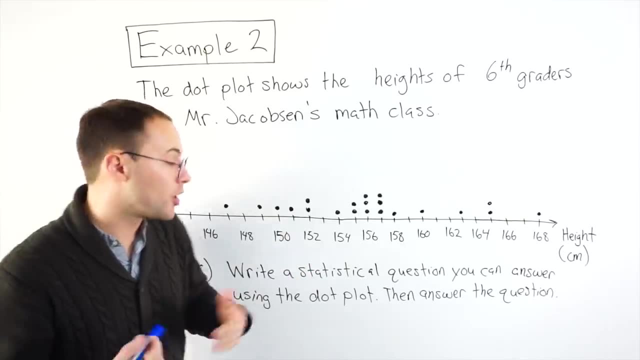 Because that's what the data was. Let's try part C. OK, finally, part C: write a statistical question you can answer using the dot plot and then answer that question. So we're writing a statistical question. It has to be about the dot plot. 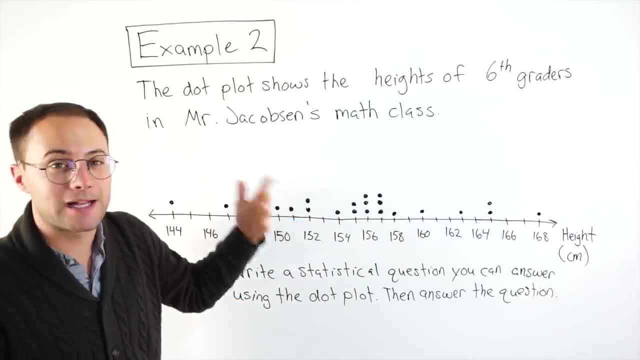 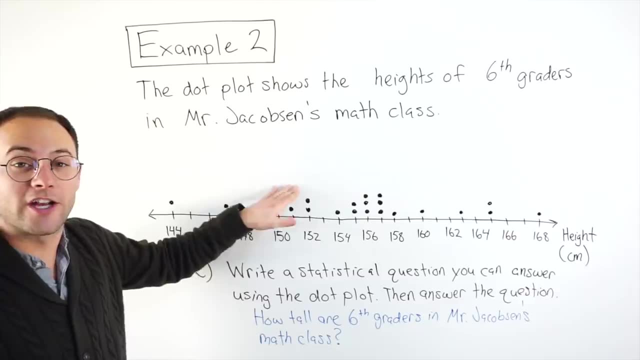 Remember this was about heights of students in my class, So maybe our question could be: how tall are sixth graders in Mr Jacobson's math class? That is a question that we could answer using this dot plot. So that's great. 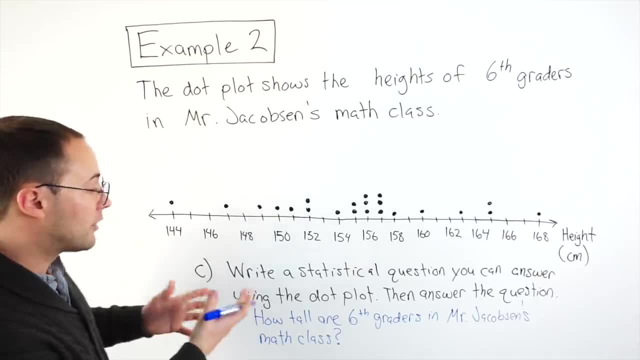 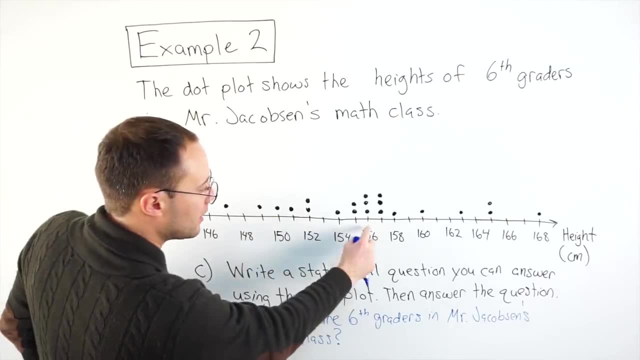 There's our statistical question and let's answer it. Well, how tall are most sixth graders in my math class? If you look, we have two peaks right here: There's 56 and 57.. By the way, you may have noticed, I didn't label every single. 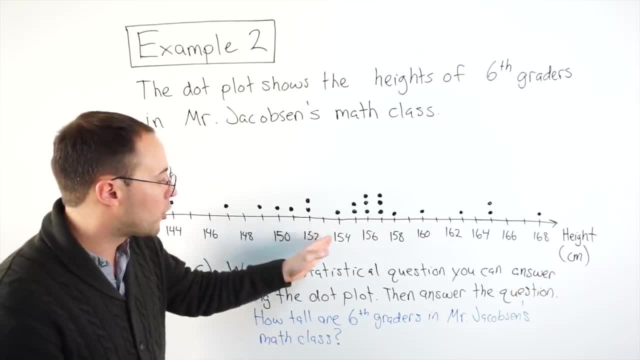 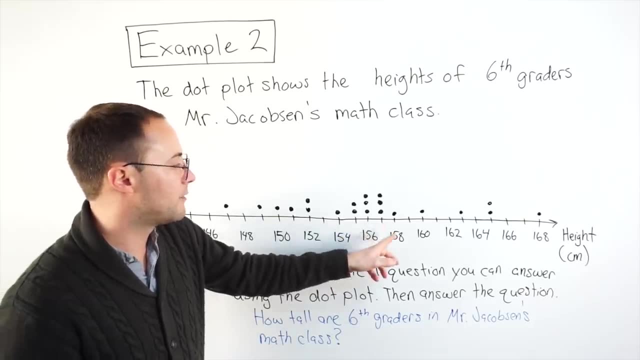 every single dash. but if you notice, I'm going by the same amount. So 152, that would be 153,, 154,, 55,, 56,, 157, 158.. That's fine, you can do it that way, just be consistent.